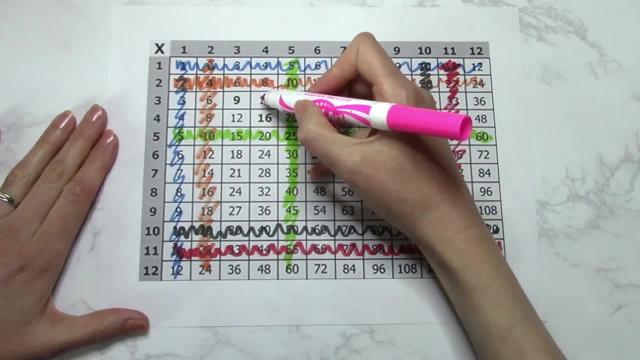 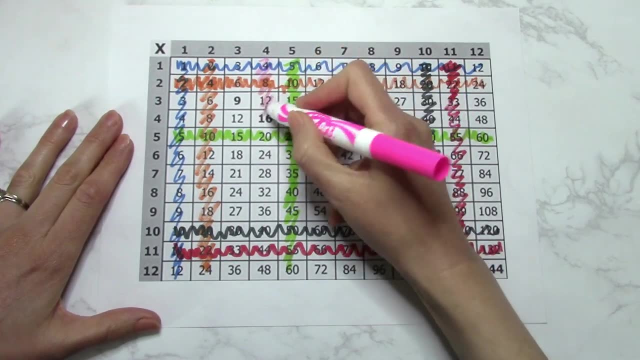 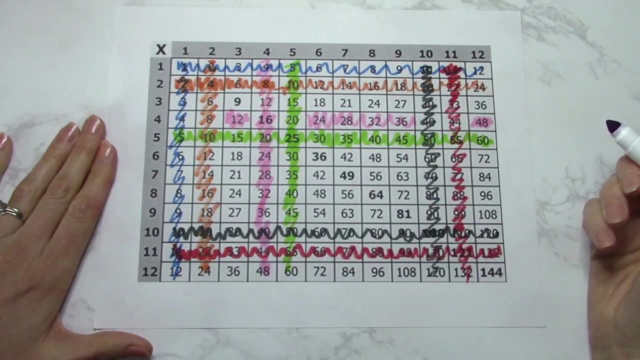 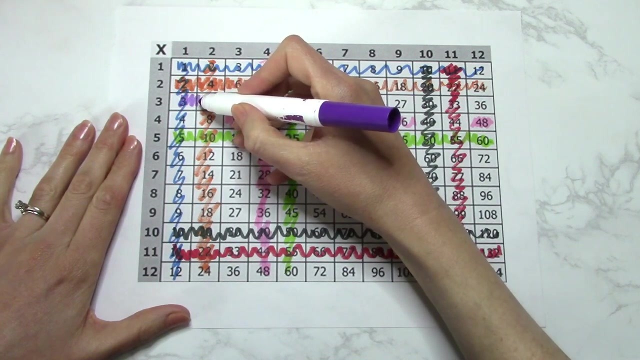 multiply it by 2s. So 2 times 3 is 6.. Multiply that by 2. And we get 12.. So 4s are pretty much like the 2s. Now 3s here can be a little bit challenging. But if you can count by 3s, 3,, 6,, 9,, 12, then you can. 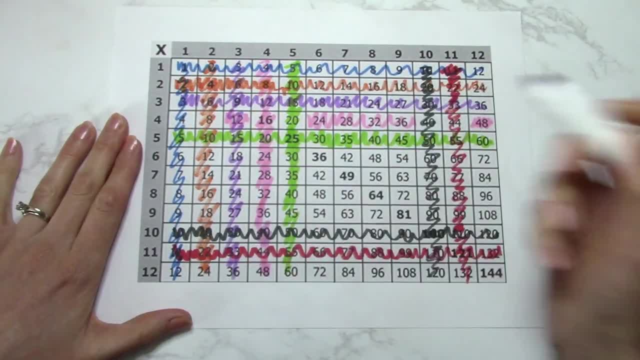 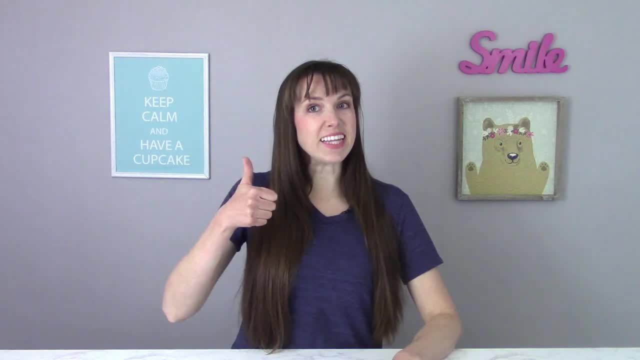 get a hang of it more or less. Look at this. We have covered so much of this board. Now, if you'd like to see more videos like this, definitely give it a big thumbs up. Now here's a trick for 12.. 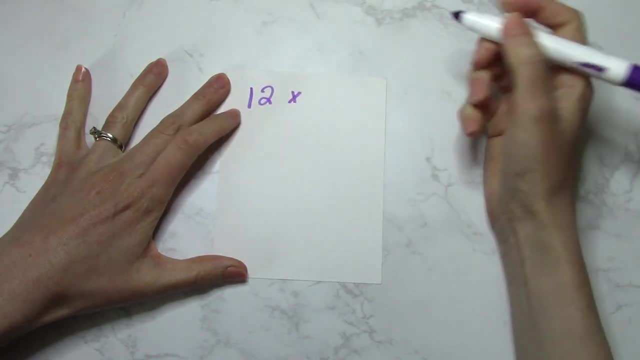 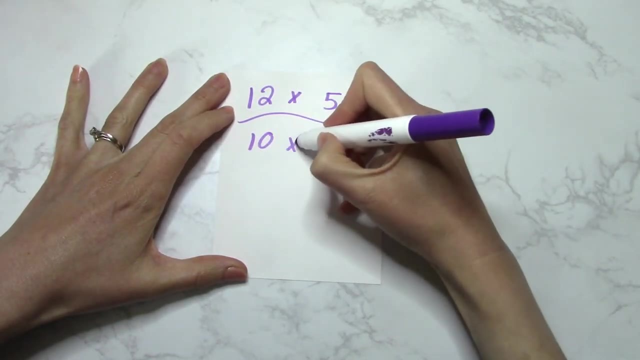 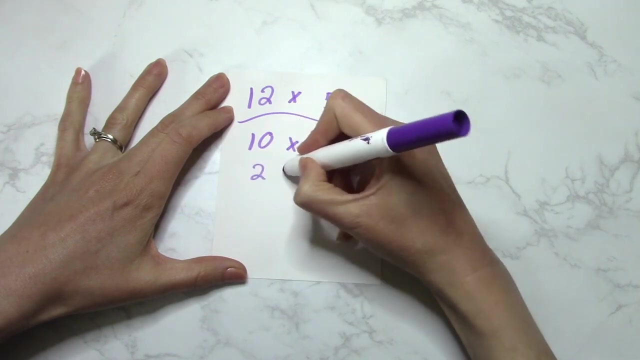 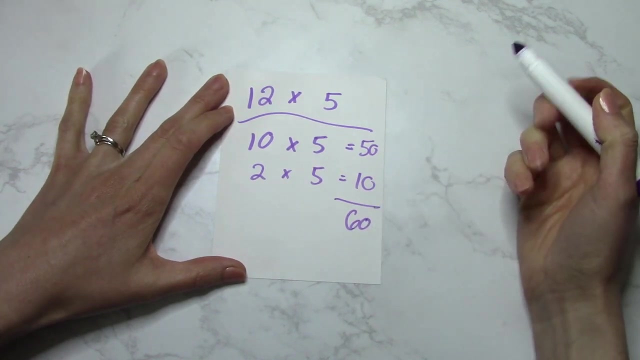 Let's say I want to go 12 times 5.. Well, I can just basically take 10 times 5,, which I know is really easy- 50. And then 2 times 5,, which is 10. So my answer is 60. So, really, with your 12s. 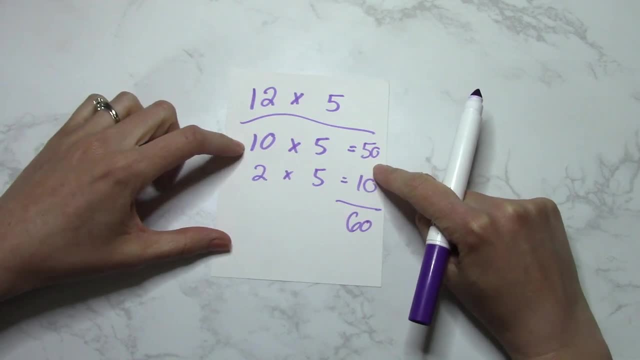 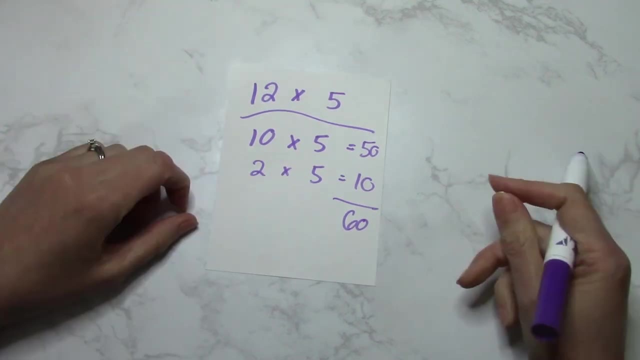 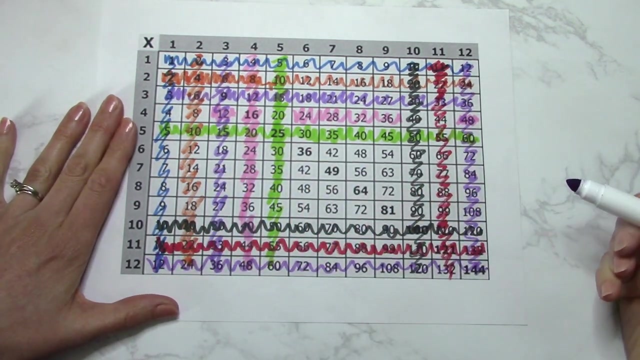 just take 10 times the number, which is easy, and 2 times the number, And then add them up together. But then of course you can always use your handy calculator. So there goes the 12s To do the 9s. I want you to put your hands just like this. Now, let's say I 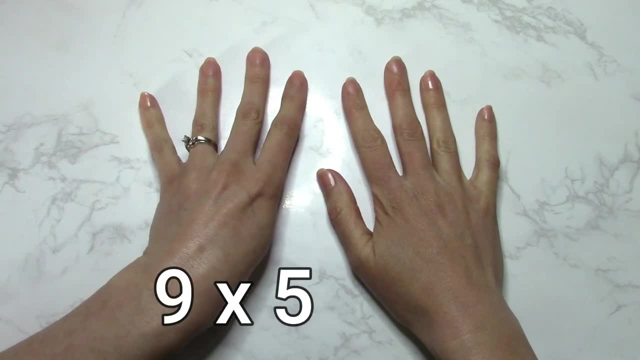 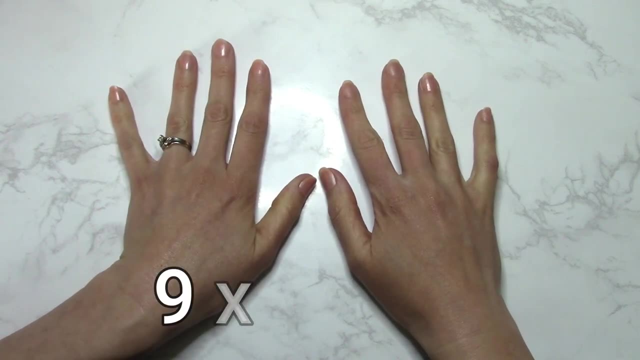 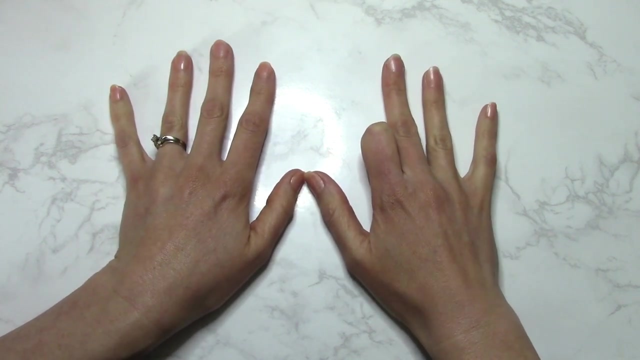 need to go 9 times 4.. Tuck in your fourth finger And the answer is 45. Let's try another one 9 times 7.. Put in your 7.. Put in your 7th finger And we have 63.. Now notice that all these numbers added up together do equal. 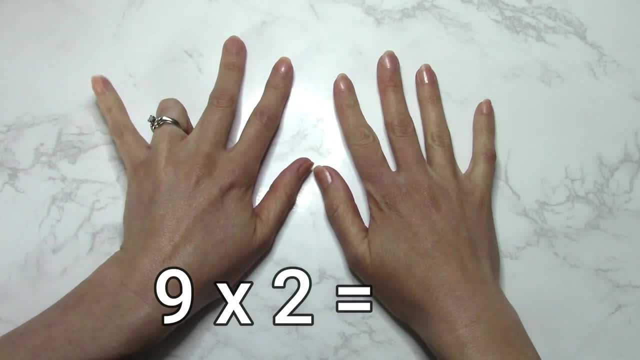 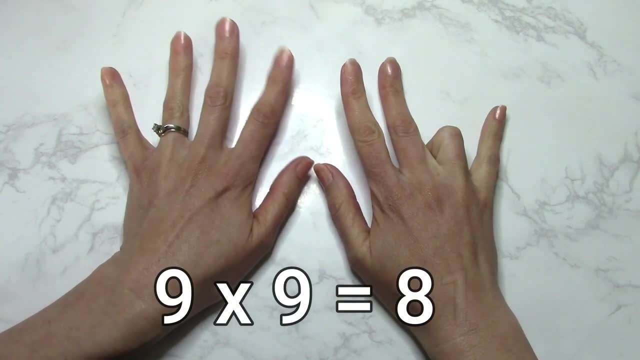 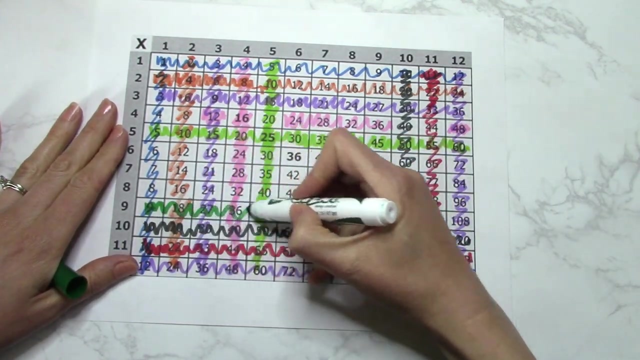 9.. But let's try another one: 9 times 2. We have 1 and 8. So the answer is 18. 9 times 9.. Tuck in the 9th finger, We have 81.. Now, whoever said we couldn't multiply using our fingers? There go the. 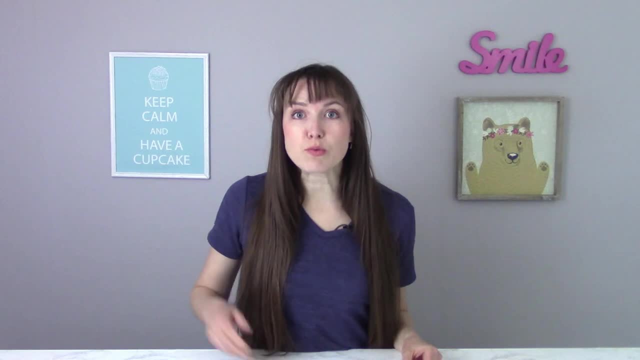 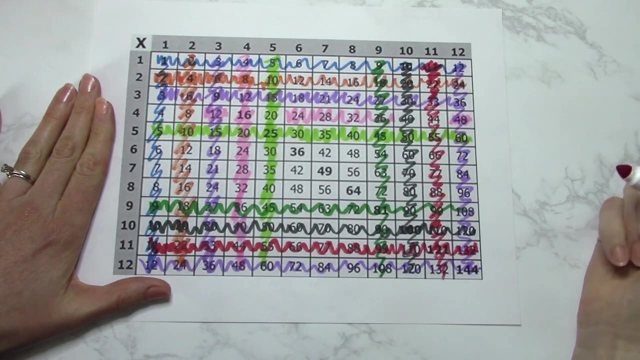 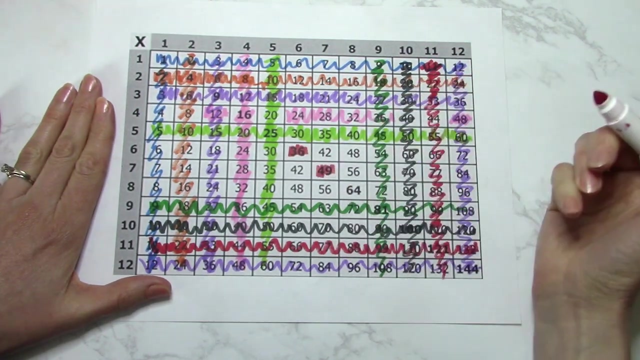 9s. 9 times 8 is really blue because it's an old 72.. Now most people tend to know what a number squared is, or a number times itself. So here, 6 times 6 is 36.. 7 times 7 is 49.. 8 times 8 is 64.. 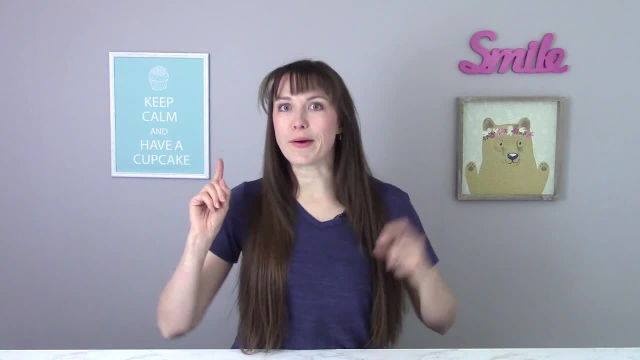 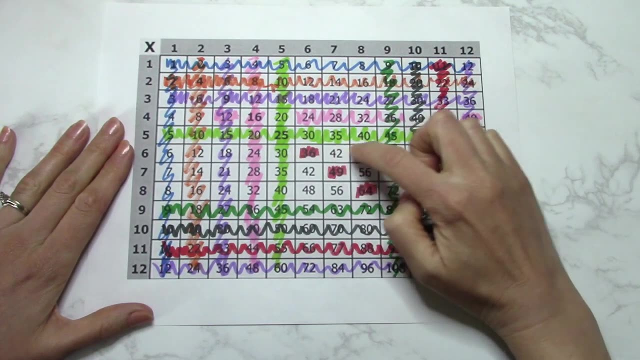 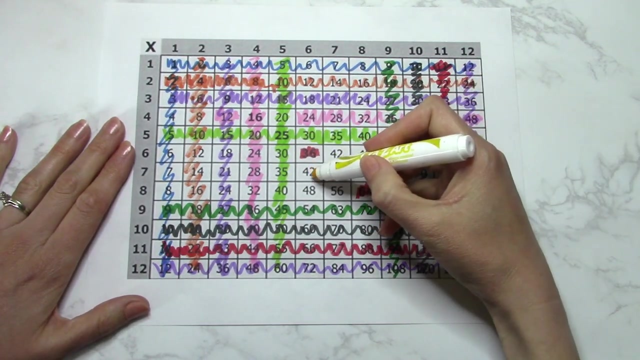 I dropped 8 and 8 on the floor, picked it up, Now it's 64.. Now we started with this whole thing: 144.. And look, now we only have 1, 2, 3, 4, 5, 6.. But wait, isn't 6 times 7: 42 and 7 times 6: 42?? 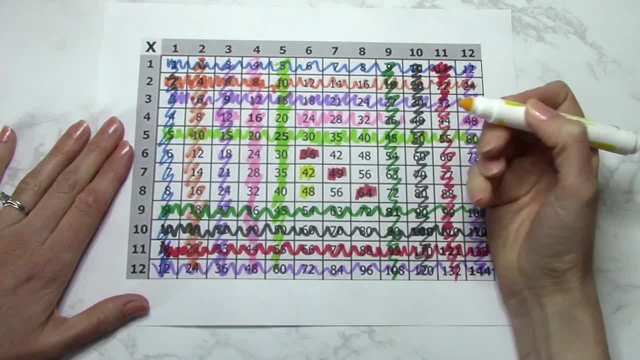 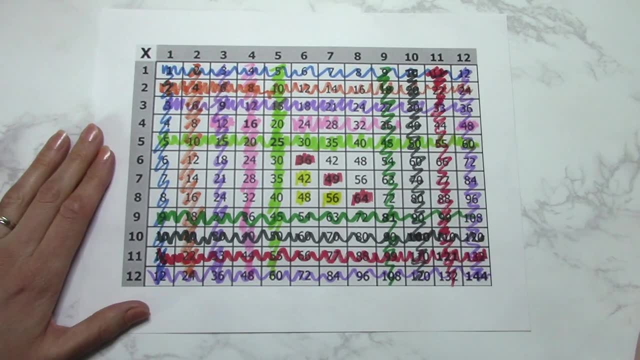 Notice we can get rid of a couple more, because 6 times 7 is the same thing as 7 times 6.. 8 times 7 is 8 times 6.. So really, most of these you understand and you've got these, Except for these. 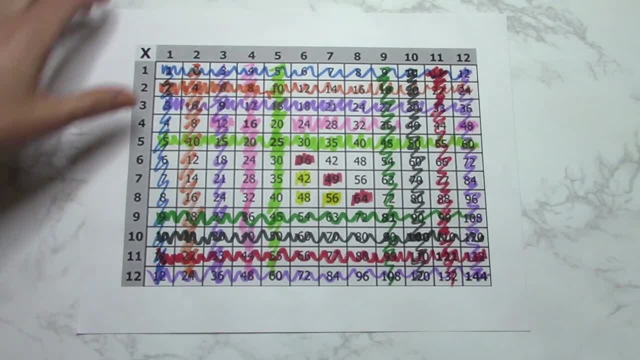 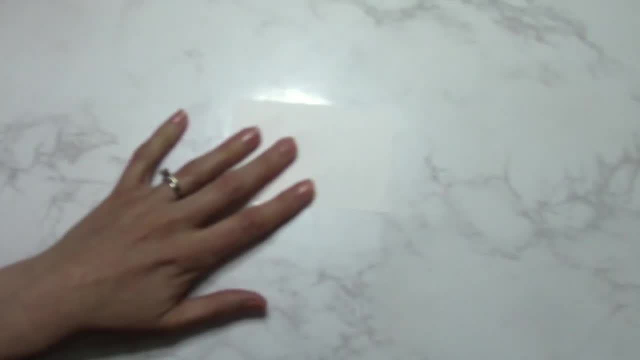 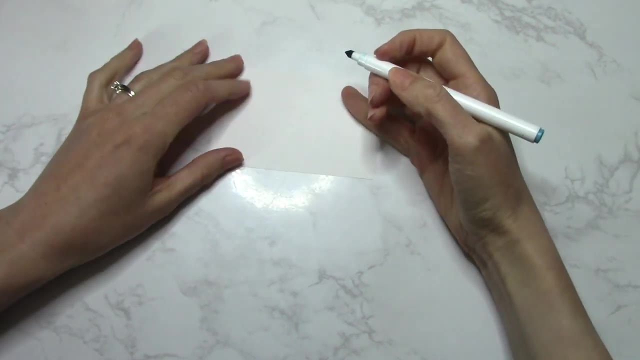 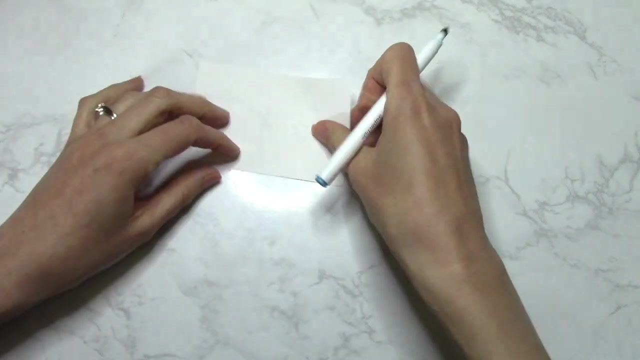 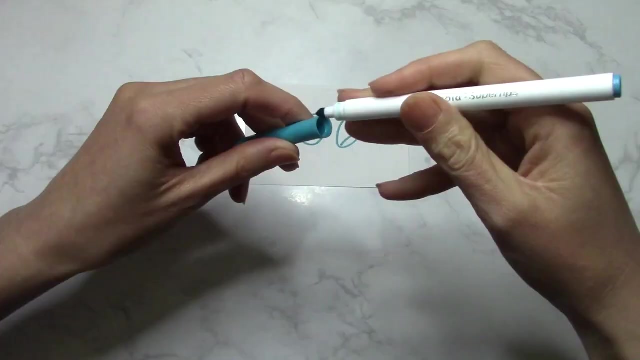 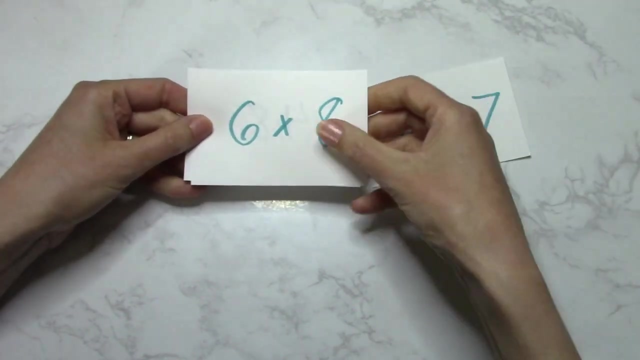 three right here. So we're going to make note cards All right, 6 times 7.. Flip it over 42.. And now I take these note cards and quiz myself Quick: 6 times 7.. 42. 6 times 8.. 48. 7 times 8.. 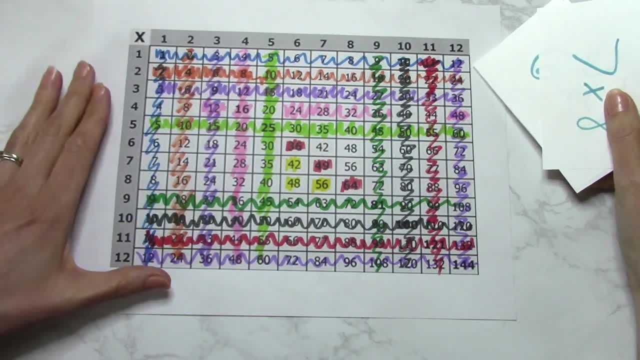 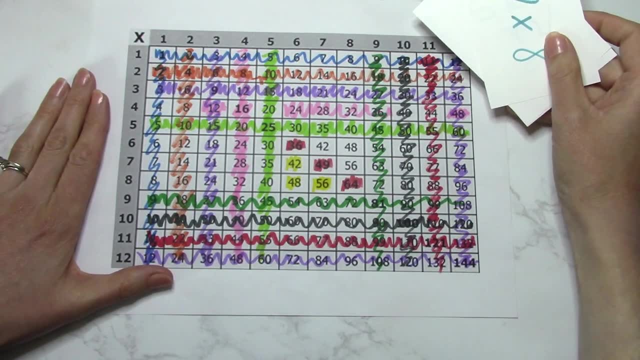 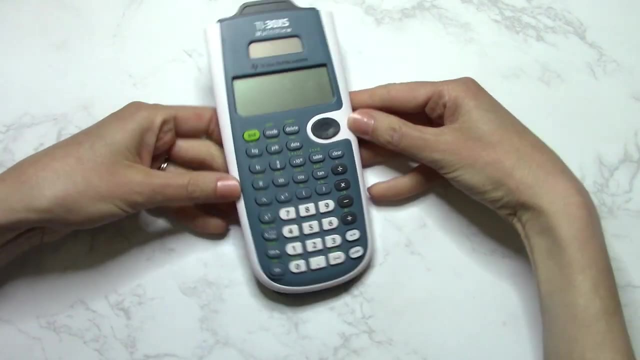 56. I hope that this multiplication chart with our couple little note cards really helps you and makes you a little bit more confident in your multiplication. Now remember, if you have multiplication down, you've got division down too. Now, if the numbers get too big, 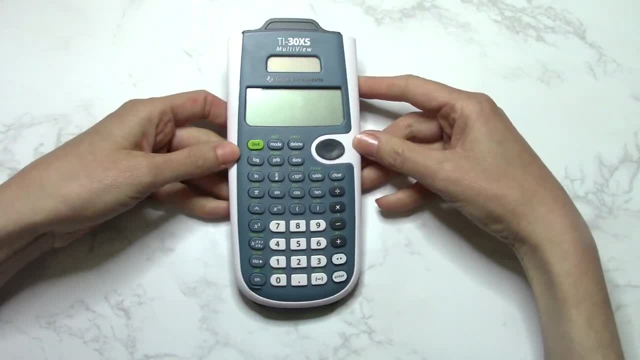 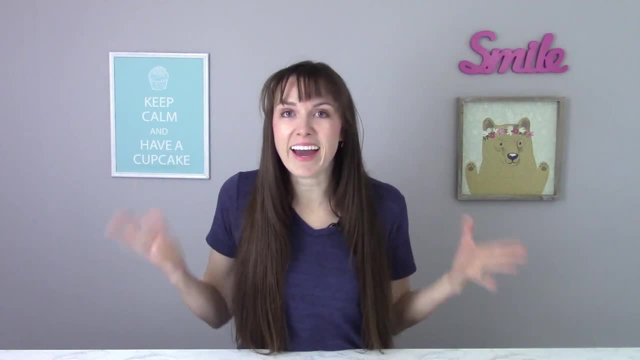 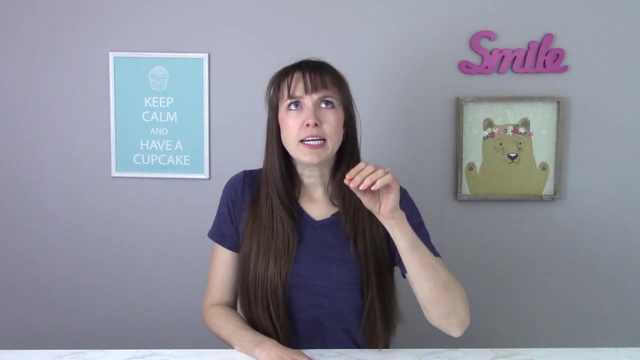 remember you have your trusty calculator that is always there to help you. Comment below if you have any multiplication, addition, subtraction Or any math hacks that can help us out. Thank you for sticking to the end of the video. I hope that you have a beautiful day and remember.